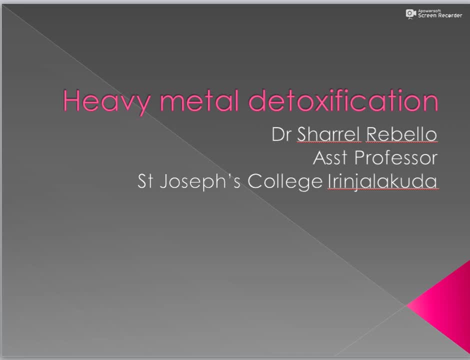 I would like to talk mainly on heavy metal detoxification, or what are the heavy metal bioremediation strategies? Of course you can include the matters which have been discussed commonly in the bioremediation for heavy metal also, But now I am trying to be a little more. 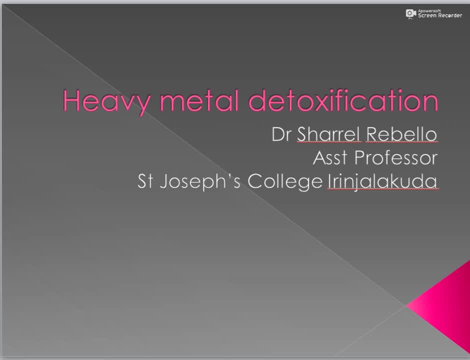 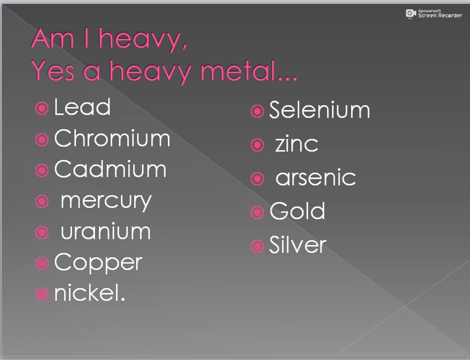 specific for the heavy metal detoxification methods. Now, what are heavy metals? Of course, heavy metals are those metals which are considered to be of high molecular weight, And these could include various methods. Now, for example, lead, chromium, cadmium, mercurium, mercury, uranium, copper. 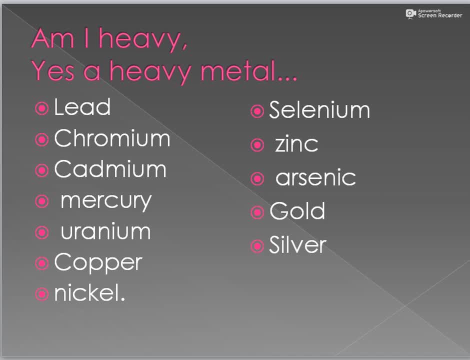 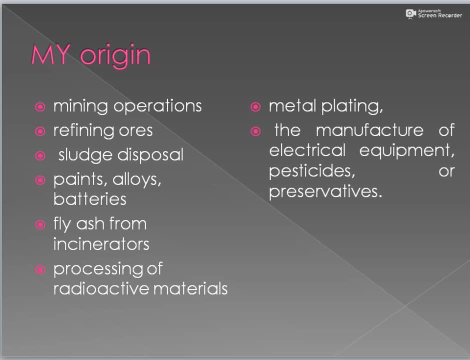 nickel, gold, silver, arsenic, zinc and selenium. These are all coming under the category of heavy metals. And where do these heavy metals come from? They can be obtained from different ways Now: by mining operations, refining ores, or when you do a sludge disposal from the panes. 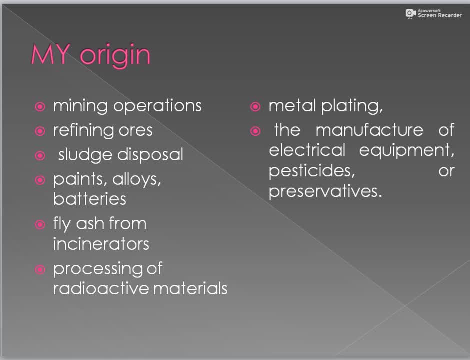 you can find it in the CRP system. Of course, for the mining operations, you can get these heavy metals by mining the oil, such as lithium, hydrogen, copper, copper, copper and sulfur, and some of these are called a bioremediation method. So here are some of the methods in which 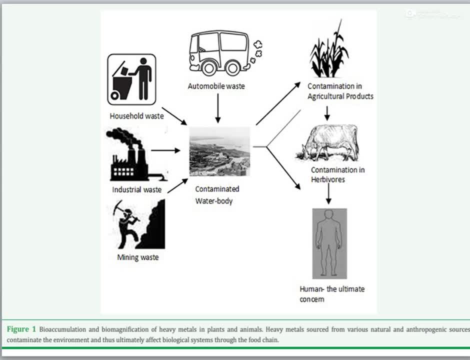 you can find those heavy metals Now, if we take the example of these hydrofoil batteries which we use, the fly ashes from incinerators or while the processing of radioactive materials, metal plating and the manufacture of electric equipments, pesticides and preservations- all of these would result in the formation of heavy metals. And these heavy metals which we use in different industries would sometimes get bioaccumulated. If we take the example of the solid metal tank, it is a highly bioaffiliated material. Do you know how to extract the lead on the solid metal plant? This is an cities of earth, that is, the complete body of solid metal. 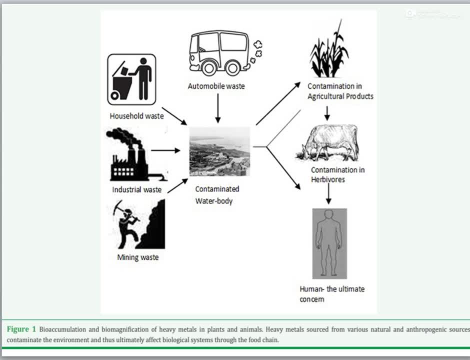 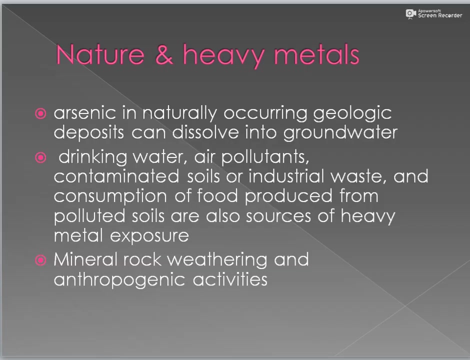 bioaccumulated and biomagnified in the plants as well as in the animals. and of course, when we consume the plants as well as the animals, they also get accumulated in within the human body too. So the remediation of heavy metals becomes very much relevant. 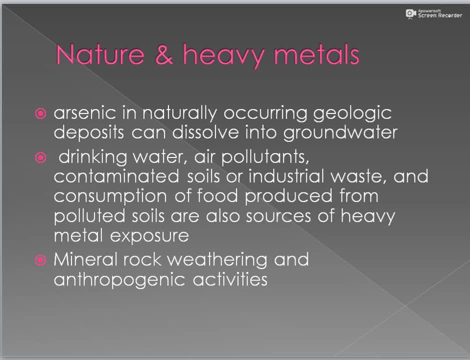 What are the nature of these heavy metals? we will just have a look. Arsenic, in naturally occurring geological deposit, can dissolve in ground water, drinking water and air. pollutants, contaminated soil or industrial waste and the consumption of food produced from polluted soils are all sources of heavy metal exposure to us. 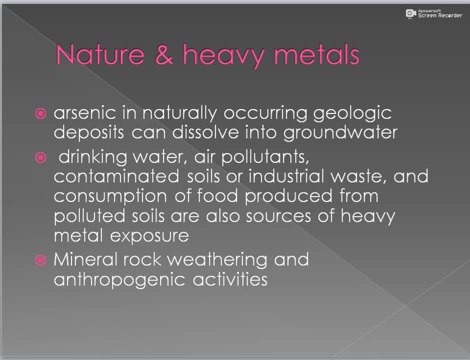 Now, when you have a mineral rock weathering, or by various other activities, when you have a heavy metals happen to come into the environment. they find their way through the drinking water, through the atmosphere, through the soil, into the plants and from the plants they can. 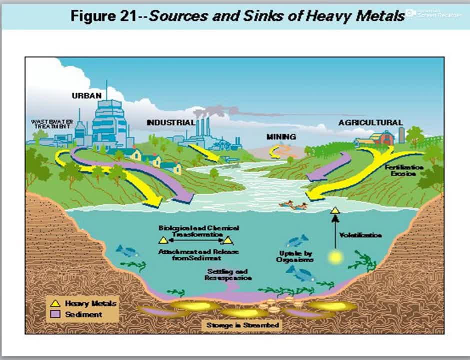 come to the animals and to the animals they can directly come to the human beings also. So all these activities, the urban activities, the industrial activities, the mining activities, the agricultural activity, the fertilizers which flow which we use, they all in that. 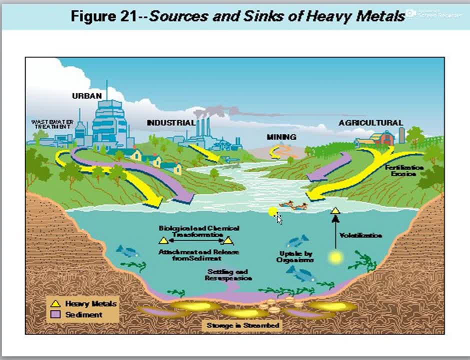 also the heavy metals happen to come into the environment, They are all coming and they happen to flow into the water along with the sediments. they will come and accumulate in the water bodies and, of course, this water body can be used as a water, as a source of water for the plants, and the plants in turn take it and, as I mentioned, 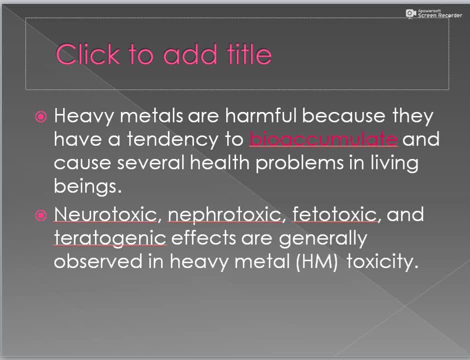 earlier. bioaccumulation and the biomagnification can happen. Hope so you remember what is the difference between the bioaccumulation and the biomagnification. Bioaccumulation is the occurrence of a xenobiotic extensively in a particular organosome and biomagnification is the step in which it increases. where xenobiotic increases. 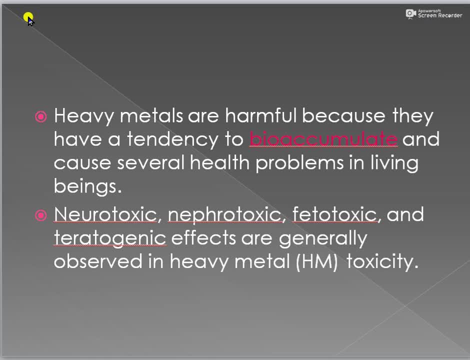 in each tropic level of the food chain. so heavy metals can bioaccumulate as well as biomagnify, sometimes by easyAUDIA, CHOPPING and even CO Churches of Logic. so having a squeeze ideia than you can use, Say some cases when they are being left in the environment and the accumulation of 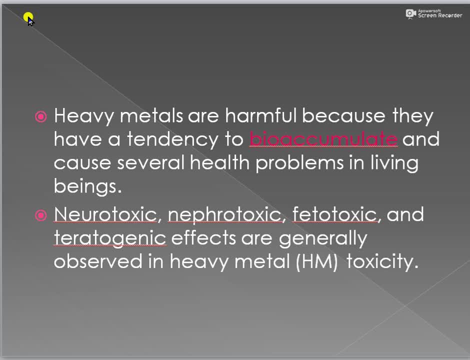 these heavy metal, heavy metals within our body could leave that neurotoxic, nephrotoxic, fetotoxic and teratogenic effects, as observed now. what do you mean? be now? neurotoxic, that is, your nerves are being damaged. nephro, your kidney is being damaged. fetotoxic, the fetus is teratogenic, cancer generating effects. so 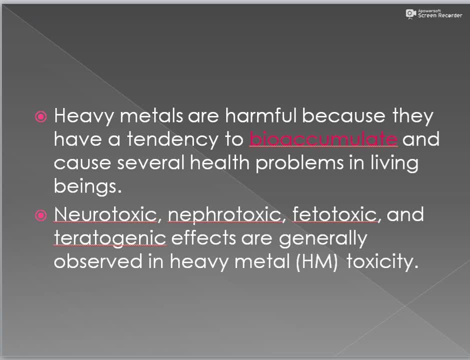 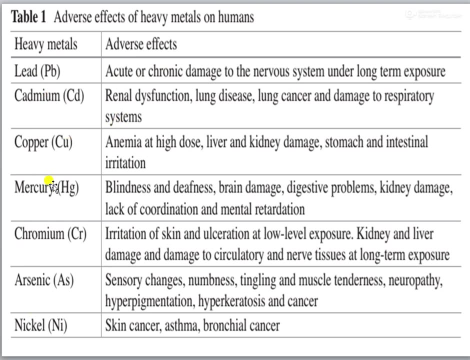 all these could be resulted as a result of the heavy metal toxicity. so let me just show you some of the effects, of some adverse effects of the heavy metals. now, lead, as I have already discussed with you, lead poisoning it is which it is a frequent contaminant in the plastic toys which children use. the yellow color: 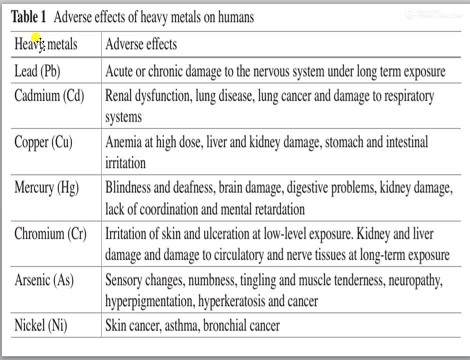 of the plastic toys which children use, the yellow color of the plastic toys ones. they are highly contaminated with the lead, so they it could cause acute or chronic damage to the nervous system under long-term exposure. cadmium- cadmium could cause defects in the renal dysfunction. renal means kidney failure. 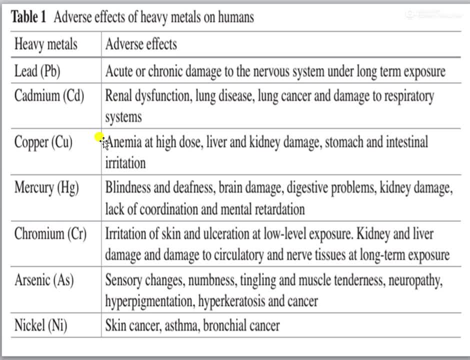 lung disease, lung cancer and damage to the respiratory system. copper- copper- it can cause anemia at a very high dose. liver and kidney damage, stomach and intestinal air irritation. mercury- now where is mercury found? mercury is: we use mercury in the, in the thermometers home. so you remember? it's just I just said, but it's a liquid. 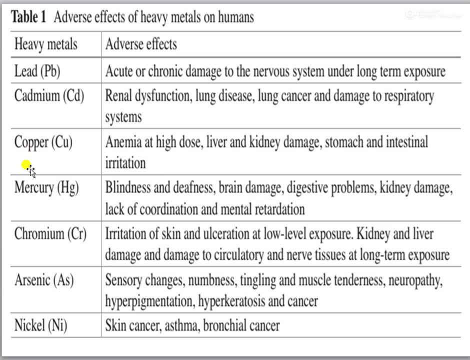 metal which we have. so the exposure to mercury can cause blindness, deafness, brain damage, digestive problems, kidney damage, lack of coordination and mental retardation. chromium: chromium is another heavy metal. it can cause irritation of the skin, ulceration of a lower level exposure, even at lower level exposure, and the kidney and the liver damage. 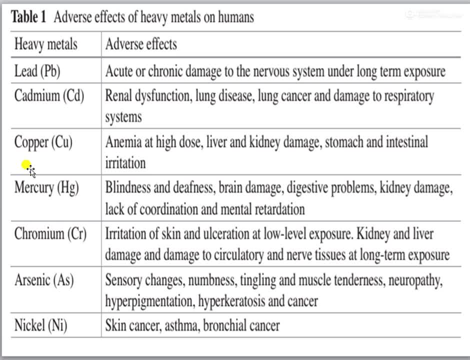 the damage to the circulatory in the nerve tissue on long-term exposure. and we have arsenic, which will cause sensory changes, nickel, which causes skin cancers, asthma, bronchial cancer, etc. now we are self know that the incidence of cancers and neurological diseases, as well as kidney failures, are being found to be very high in the liver and liver cancer and liver. 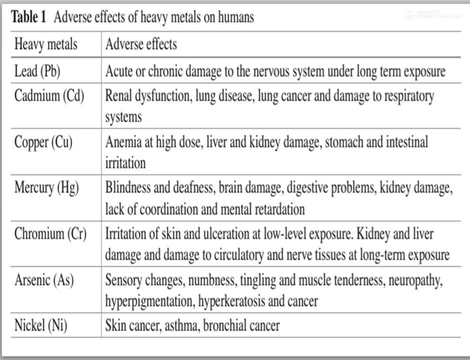 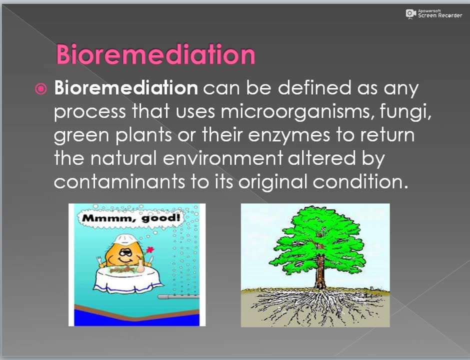 disease, and the entire nowadays. so what are the reasons for it? you can find out whenever all these chemicals happen to enter your body. they are a burden to your body and that could lose them to adverse effects. now, of course, the term by remediation is quite familiar to you by now. it's 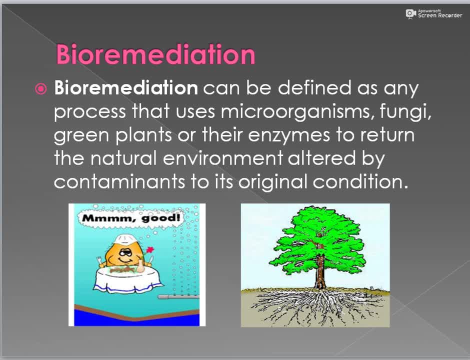 but nothing. any process when you use microorganisms, fungi, as well as any green plant, or their enzymes to return, or it can be any biological agent. when you use one chemical to scale and when you use them or the enzymes to return the natural environment altered by contaminants to. 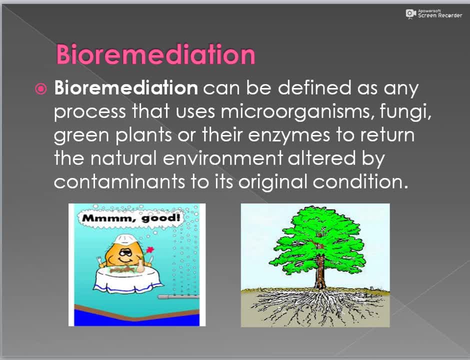 its original condition. So what does it mean When you use any biological agent to remove or degrade the xenobiotic that is referred to as a term called bioremediation, and the aftermath of that is what You will try to make the environment into a natural condition, as it was So in a 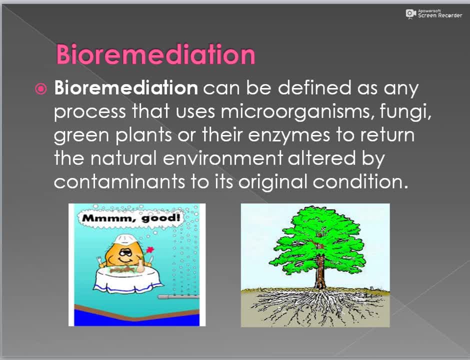 polluted environment you have lots of xenobiotics which will harm it. So by the process of bioremediation you use microbes, fungi or even sometimes green plants and their enzymes, because they are also biological agents. You might use them and convert these pollutants into less toxic. 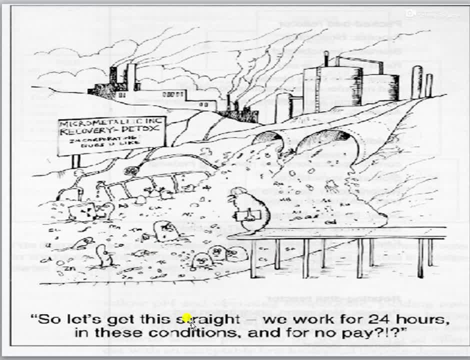 or harmless compounds. So this is just a cartoon. So let's, these are some microbes which are depicted over here, So let's get this. We work for 24 hours in these conditions and for no pay. Of course, the microorganisms are detoxifying some of these xenobiotics and that's the commentary which we came across over here. 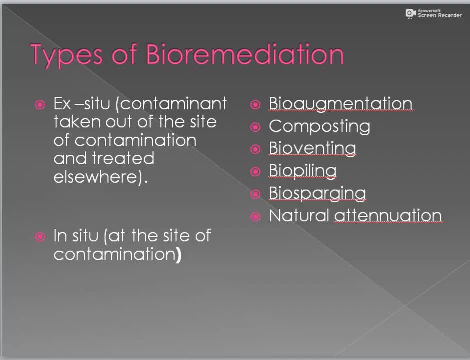 So the term bioremediation using biological agents can be carried out ex-situ or in-situ, as we had already discussed. and different terms. There are different technical interventions of them: Bioaugmentation, composting, bioventing, biopiling, biosparging, natural attenuation. Of course you can just 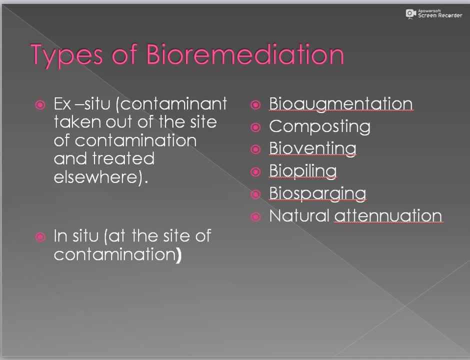 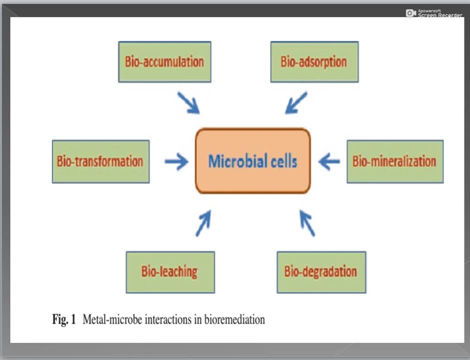 go through the videos which I had previously explained on these and what happens in bioremediation of heavy metals. Let me just tell you that, And when a microbe is coming into interaction or when it is interacting with a heavy metal, either, what it does is the heavy metal will. 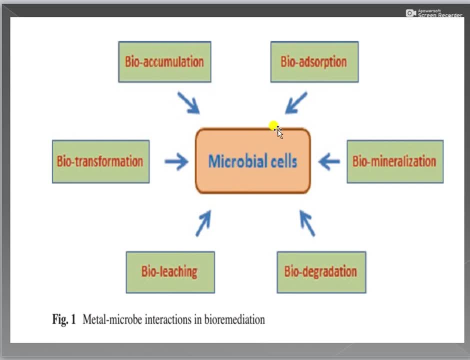 get accumulated In the microbial cell or it can do the process of bio adsorption, that is, on the surface of the microbial cell. the heavy metal will get adsorbed onto the surface or it will biomineralize it. Biomineralize it means de-gride the heavy metal and make it into break down the heavy. 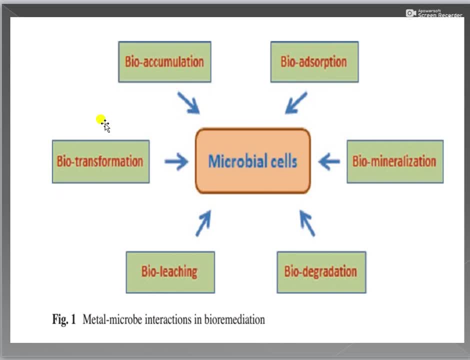 metal and make it into a small mineral, Then biotransformation, that is, converting the heavy metal containing compound into something else, Or the other one, bioleaching. Bioleaching is a process which we will be discussing in detail. It is a technique. where you are, the microbes will use the heavy metals and help us to extract. 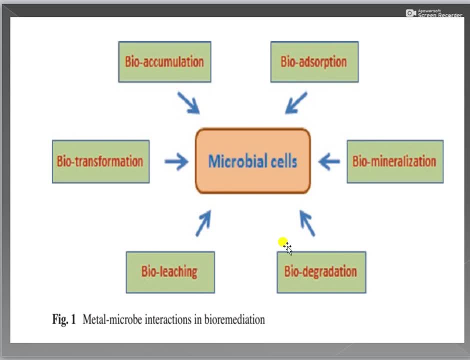 some metals and, of course, the process of biodegradation. Biodegradation is the process of breakdown of the components. So this biomineralization is the formation of producing minerals as a result of the breakdown. So all these are the processes of biodegradation. 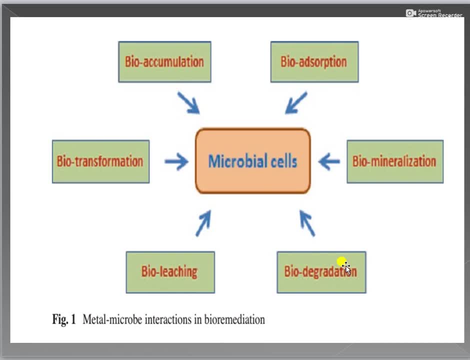 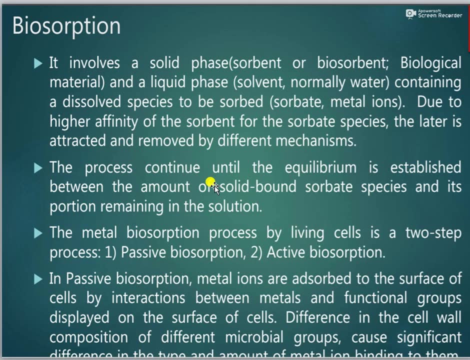 So biomineralization is the process of the breakdown of the components, So biomineralization is the process of the formation of producing minerals as a result of the breakdown of the components. So these can happen within the heavy metal detoxification. So let us talk about bisorption or bio adsorption, and this is nothing but it involves a solid 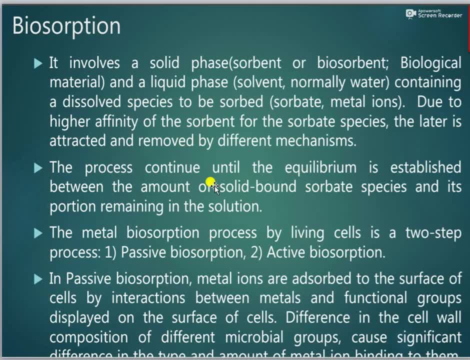 phase- For example, it could be any biological agent- and a liquid phase which will contain a dissolved species to be absorbed. That is, for example, if a metal ion is contaminated in the water, the water will serve as a liquid substance And because the sorbate substance- the sorbate is nothing which will absorb the what heavy 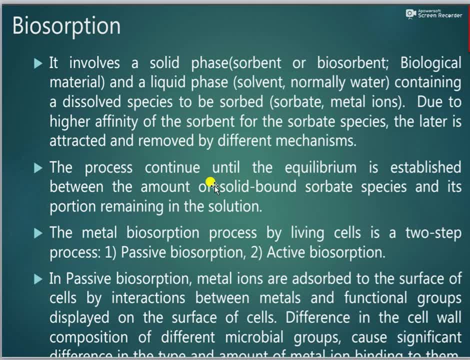 metal onto it. That will be there and the water is also being brought. and what would happen? the water, the heavy metals from the water will be absorbed onto the biological agent, and this can be done using living cells, either by passive absorption or active absorption and passive. 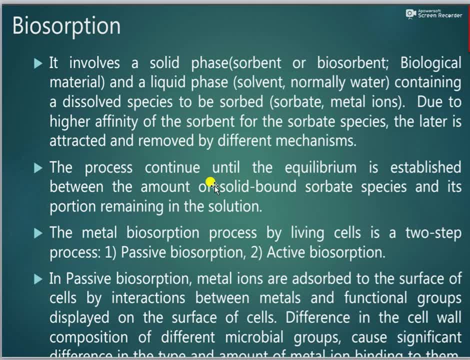 absorption: the metal ions are absorbed onto the surface of the cell by interaction between metals and the functional groups displaced on the surface of the cell. And you just have to remember the concept that from a liquid phase the heavy metals are being absorbed onto a particular substance. 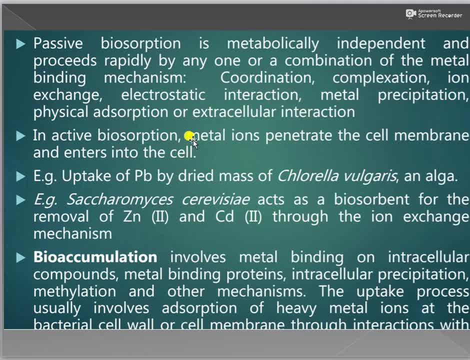 So in passive absorption it is a metabolically independent process and what happens? it can proceed rapidly. It can be done by any or one of the combination of the metal binding. you do not have to worry about it. It just remember that it can active happen either actively or passively. 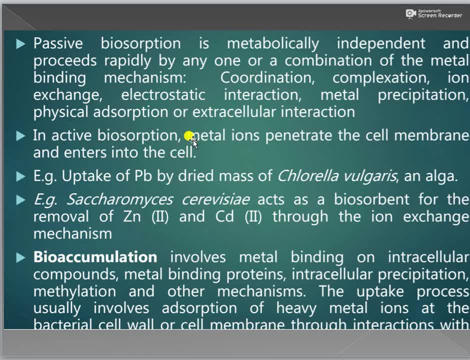 In active absorption, the metal ion penetrates the cell membrane and enters into the cell. In passive absorption, along with certain other substances, the metal is also getting absorbed Now, for example, like coordination, complexation, ion exchange, electrostatic interactions or metal precipitation, etc. 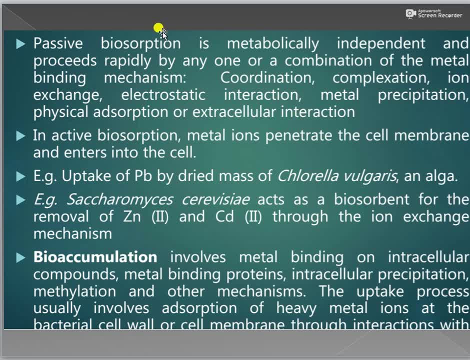 By that, passively, the metal gets absorbed. and one of the inactive case what happens? the metal is penetrating into the cell membrane and entering into the cell. Now, an alga called Chlorella vulgaris. Chlorella is an alga which we can also eat, which we consume. 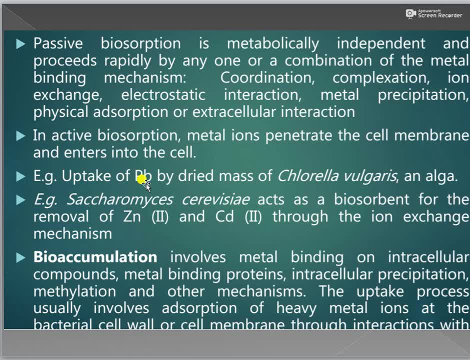 So some species of that, now Chlorella vulgaris, it is being used to take uptake of lead. Saccharomyces cerevisiae, Which is an adsorbent algae. Saccharomyces cerevisiae, Which is an acid. Saccharomyces cerevisiae is. you can also take uptake of lead. 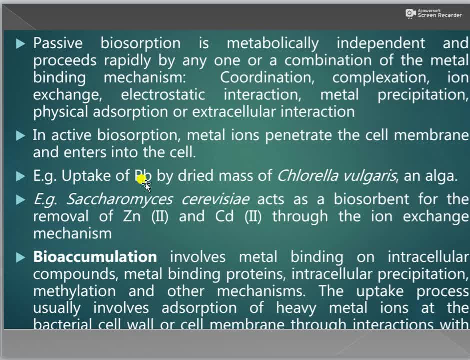 Saccharomyces cerevisiae, can be oxidised. It is an acid and it can also be oxidised, So it is an acid that require some amount of iodine and that is why, again, you can say that this is an acid which has a lot of iodine and that is why you need to take it uptake. 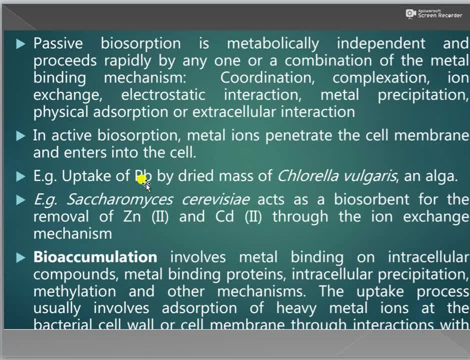 of iodine, Now an oxidation process, And an oxidation process in a cell which is in that cell is called agination process. What you can see in an agination process is that you can see that it can act on an oxygen, like it is that of zinc and cadmium, through ion exchange mechanism. 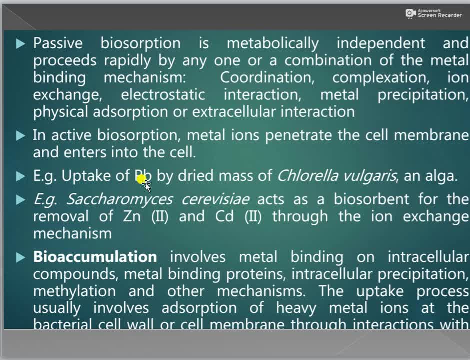 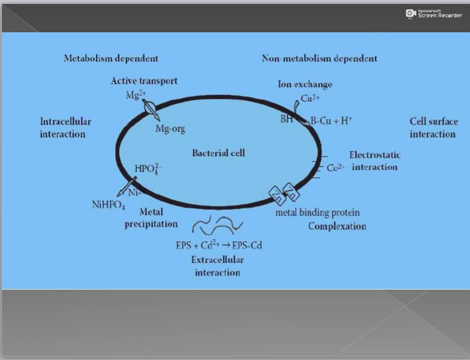 And you can see that the process of bioaccumulation can also happen within these organisms, by the process, when they are bit treated with heavy metals, or we already know what is bioaccumulation because we have already explained it in the previous videos. so the bacterial cell, okay, it can undergo different methods, like by active transport, the 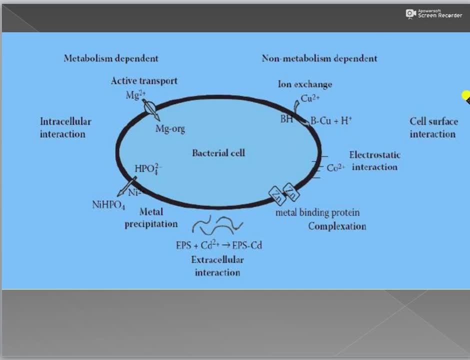 heavy metal can go inside, or by ion exchange. it can. that is, instead of the heavy metal. it will. it will take up the heavy metal instead of some other one. now copper is taken and a hydrogen has been replaced out- that is an ion exchange method- or by electrostatic interactions. now, for example, the heavy 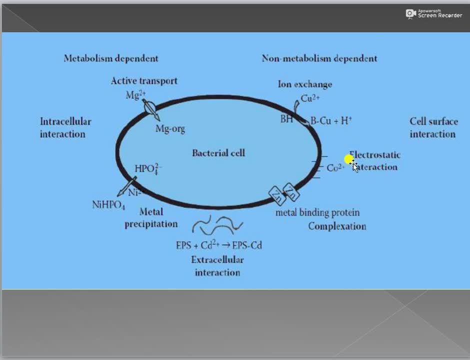 metal is having a charge and the cell will have a negative charge. so it is absorbed on to it, or by with the help of certain metal binding proteins- that time the microorganism might take it- or by extracellular interaction. for example, the bacteria will produce some extracellular produce products. okay, okay. 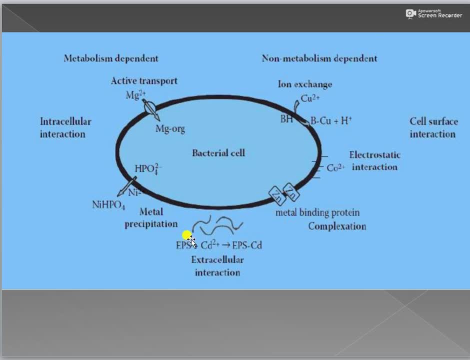 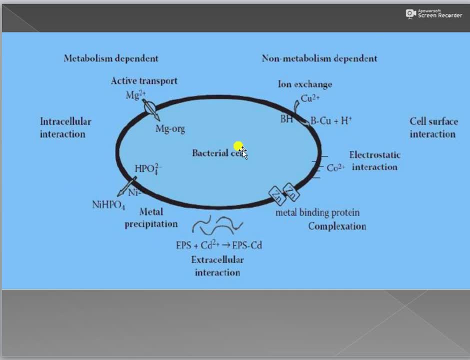 or sometimes the metal will get precipitated, so like that the bacterial cell will take up the heavy metal by different methods, either actively taking it inside, or by ion exchange, or by electrostatic interactions, or by complexation. where metal binding is not possible, proteins will play a role- or by production of extracellular polysaccharides. 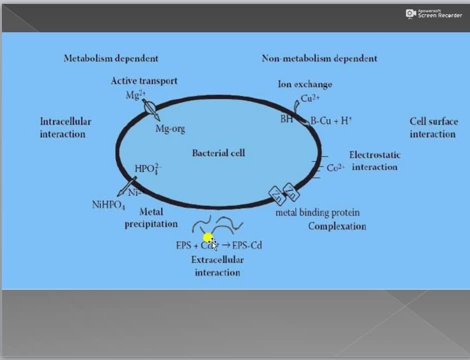 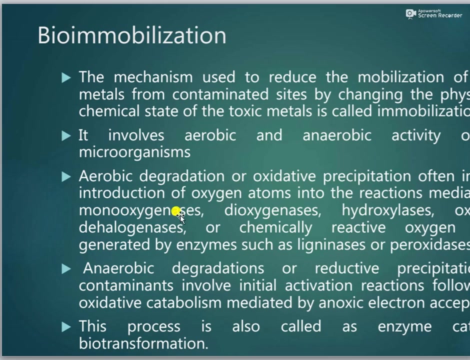 which will, or polymeric substances- sorry, extracellular polymeric substances- and they will react with a heavy metal, or the metal precipitation can happen by all these techniques. the microbial cell will take the heavy metal with it inside and in some cases you can also find a process called bio immobilization. what is that? 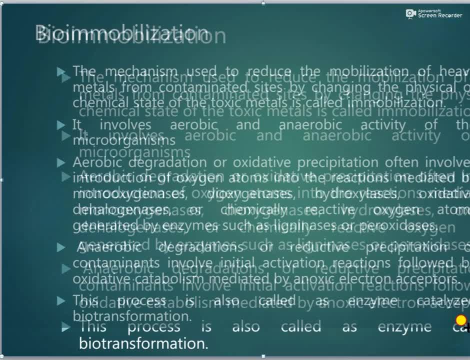 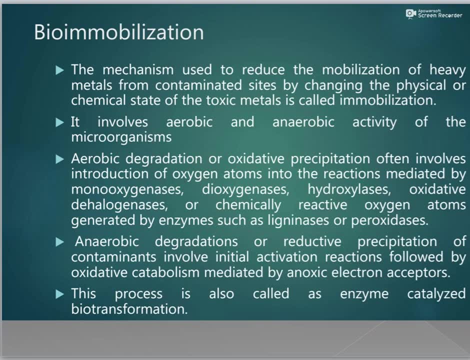 bio immobilization. what is that? what do you mean by bio immobilization? bio immobilization is nothing but a technique in which biological agents are mainly being used so that they, they will be immobilized in a particular way. what do you mean by immobilization? immobilization means trapping- okay, the bacteria or the agent which is used for. 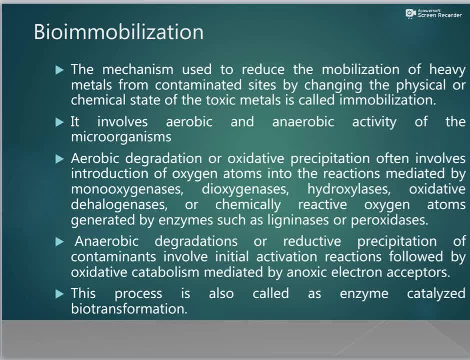 the heavy metal that is being trapped in a gel, like structure or something like that, and then they will do the process of biotransformation or bioabsorption and all that. that is called bioimmobilization. it's nothing, it's just the same thing, you know. I'll give you a simple example. you take: 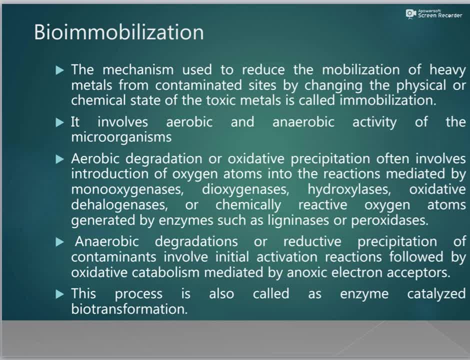 your bacteria, put it into a gel and keep. the bacteria is in such a way that it is inside the gel. it cannot move from the gel. but when I pass some heavy metal solutions through it, the bacteria within the gel will take up the heavy metals onto it and the water will. 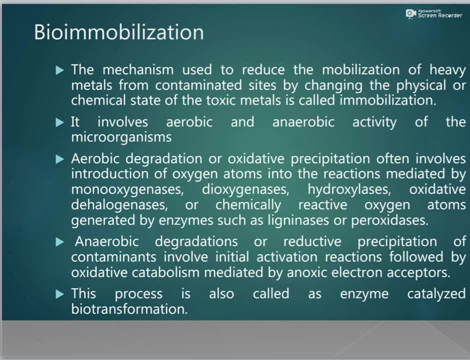 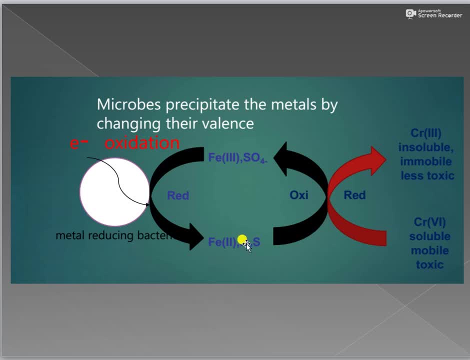 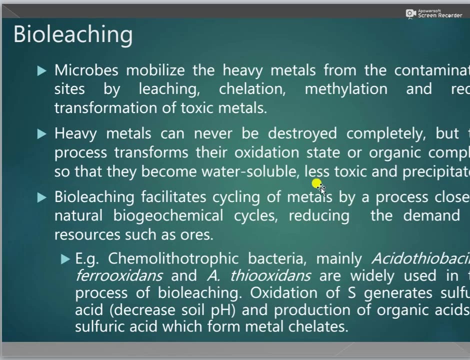 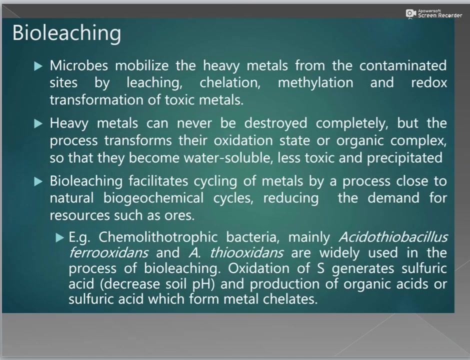 be free from the heavy metals. that is an example of bio immobilization. so that is also a way of- and this is another one where we precipitate it, because I have already discussed this technique- and then you can also use it for bio leaching. okay, bio leaching is nothing, but the microbes mobilize the heavy. 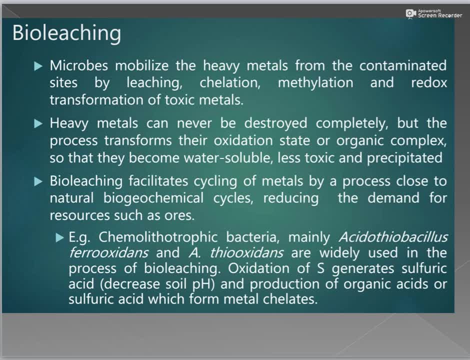 metals from contaminated. that is, they remove the heavy metals from a contaminated environment and you the metals are in such a way that they are not yet oxidized, yeah, a way that you can utilize it for others. we will be talking about that in in the next session. 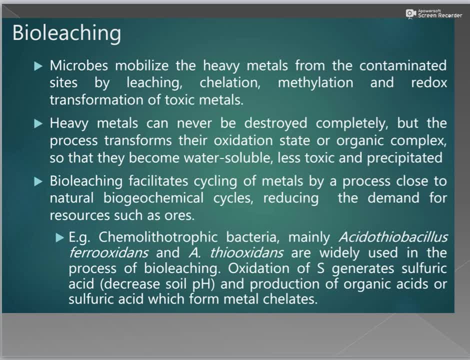 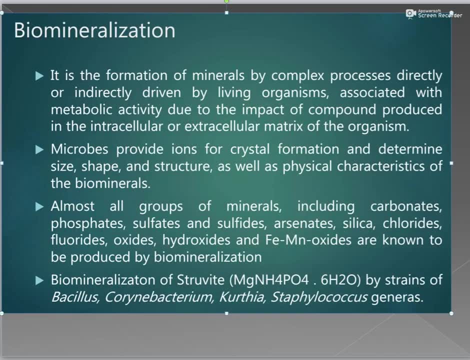 because we have a separate session on bio reaching, so that is why i am not going to discuss it right now. so, uh, you can also do the process of bio mineralization, okay, uh, it is a formation of minerals by complex processes directly or indirectly driven by the living organisms. 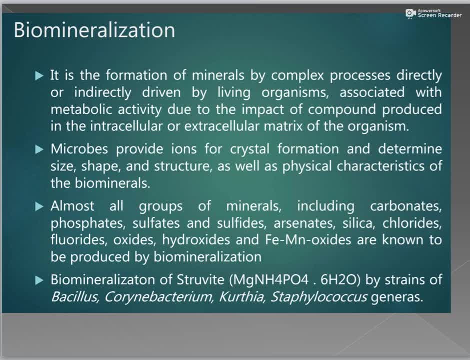 associated with the metabolic activity due to the impact of compound produced in the intracellular or the extracellular matrix of the uh organism. i had told you about eps, which is being produced by the organisms. so the organisms will produce certain uh eps, or biosurfactants or something. 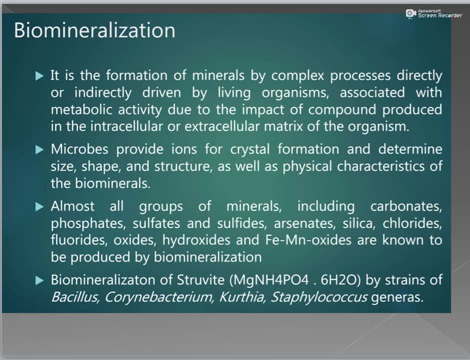 like that into the extracellular environment, or sometimes they will produce certain compounds in the intracellular environment which will help to convert these heavy metals into metal uh, into minerals- that is the process called bio mineralization- and uh various bacteria like bacillus corny, bacterium uh, staphylococcus kurtia and all that. 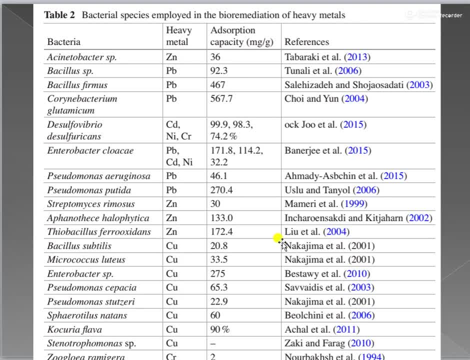 they all can do the process of bio mineralization. and these are some of the bacterial species which can be used. uh, you do remember thio, bacillus peroxidants, because that is important in bio leaching as well as in heavy metal. then corny bacterium glutamicum desulfovibrio. 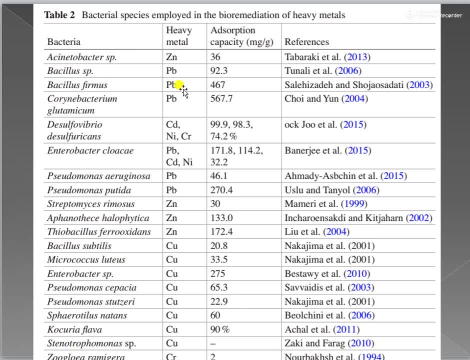 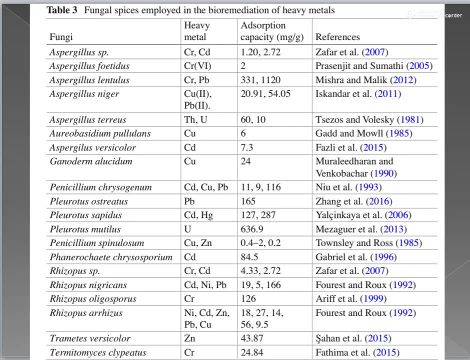 acinetobacter. these are all some of the important members which can do the process of heavy metal leaching and uh. we also do have fungal species like aspergillus uh. ganoderma pensilium pleurotus. these are all other fungus which can do the process of heavy metal leaching. 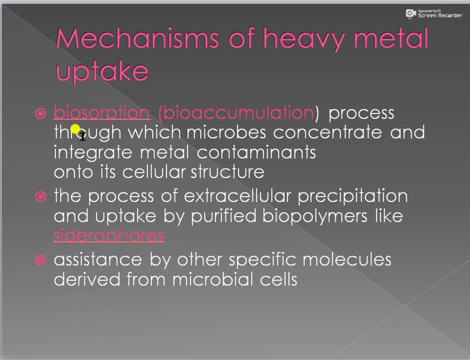 and what is the mechanism of heavy metal uptake? one was a biosorption. i told you biosorption and the bio accumulation neutral, and this process of uptake can be carried out with the help of certain polymers. now, for example, if it's a iron bearing heavy metal, you can produce some siderophores. you have learned about siderophores. 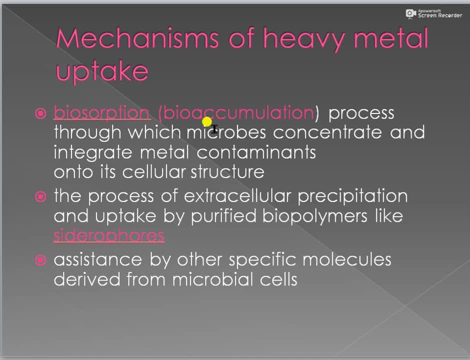 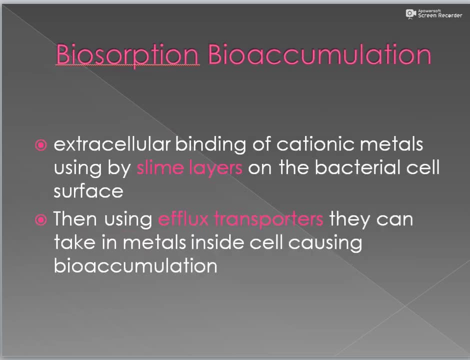 as metal uptaking proteins. these siderophores will help to take about metals. then assistance of specific molecules which have been produced by microbial cells that will help us then extracellular production of now, for example, slime layers could be there. that would help uh to take the heavy metals onto this body surface or sometimes efflux transporters. 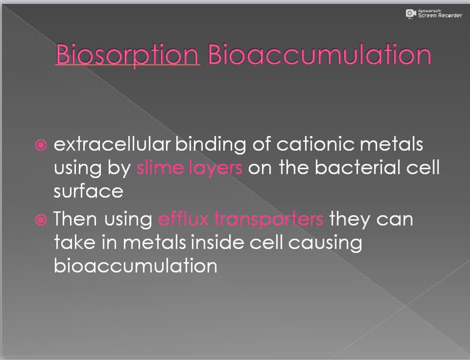 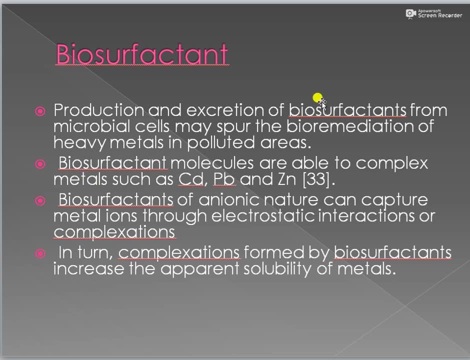 which will take in the metals inside the cell, causing the bioaccumulation. then you can have the production of certain agents called the biosurfactants. as i told you, biosurfactants are make. uh, we had discussed about biosurfactants in the oil spills. 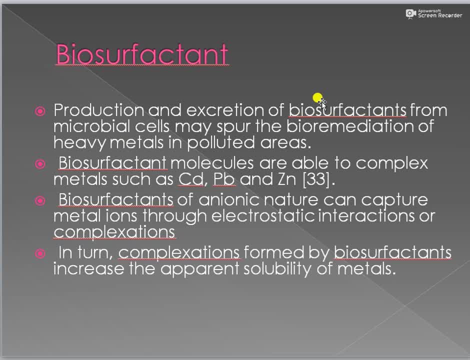 which will help to make the oil soluble in water. the same way over here, the use of biosurfactants will also help to take up heavy metals, uh, by, like, for example, titanium, lead and zinc and all. they all can be taken by using biosurfactants and they might. 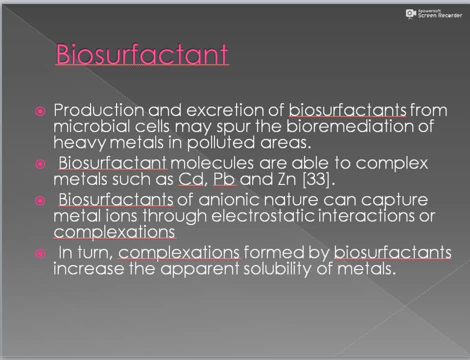 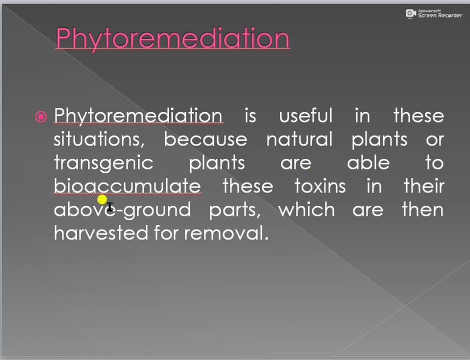 involve electrostatic interactions or complexations which will enable the heavy metal to be taken. and and of course, the next method of bioremediation of heavy metal is by using phytoremediation. the term itself is helping you to understand that: the use of plants to take up the heavy 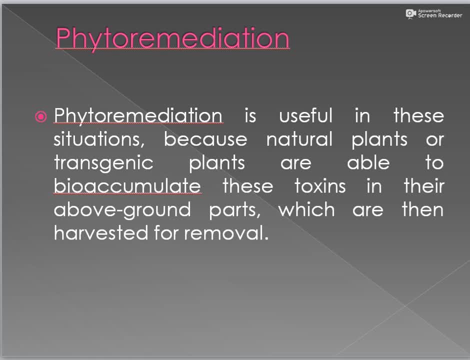 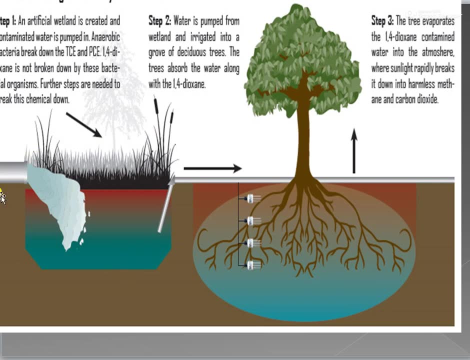 metals from the ground or from the soil can be carried out using plants, and what happens is, if there is a plant, uh and if uh through the exudates, if the heavy metal is coming into the soil, the plant roots will take up. what happens will take. 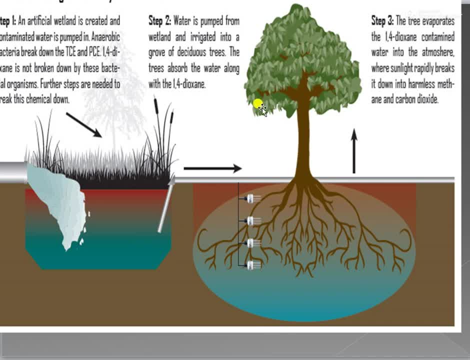 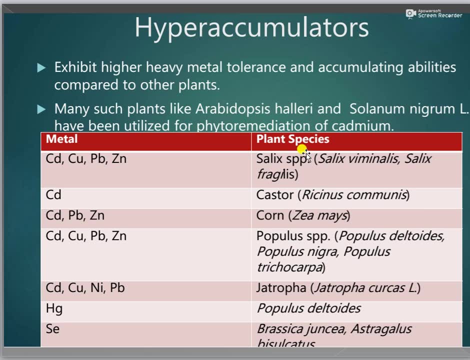 up the uh heavy metals onto it and that will get accumulated within the plant, and these are called the hyper accumulators. now, some of the uh plants have a uh what greater ability to take up heavy metals, and these are some of them, like salic species, which is 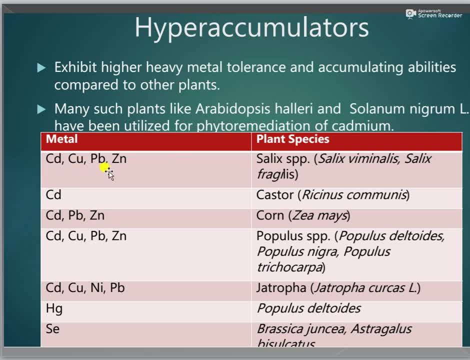 a good in taking up metals like cadmium, copper, lead and zinc. castor- uh- castor is a wild plant. okay, it is helping a white plant you know about- you can see it across the villages and all that. castor plants are just growing like that and they are capable of taking up cadmium and uh like that. 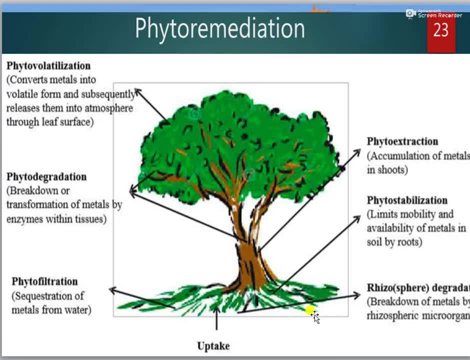 are over there. so this is a case of phytoremediation, uh, which in which the plant will take it, take it up, and sometimes phytodegradation or the breakdown will happen and uh, sometimes, uh phytostabilization will happen and uh, the rhizosphere degradation, that is, uh the degradation. 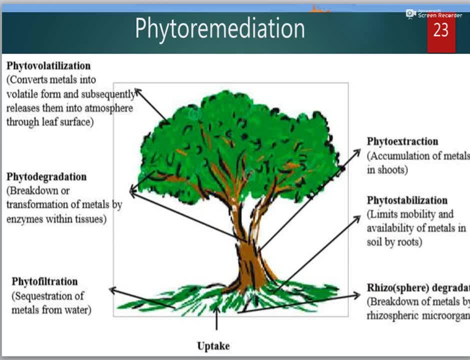 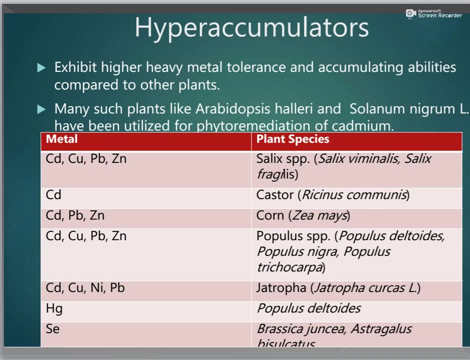 of the metals happens at the rhizosphere, or the rhizosphere is a- uh orgasms, as a rhizosphere is a which has been associated with the roots of a plant, so there also degradation can happen. okay, yeah, i have already mentioned this, and of course they do have some advantages of 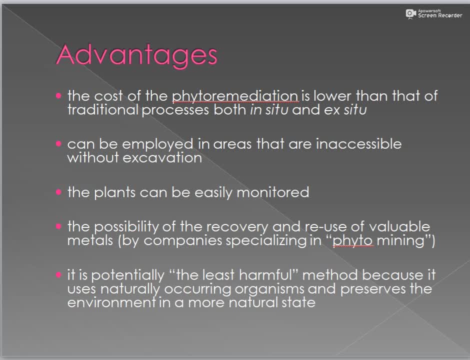 bioremediation. the cost of phytoremediation is lower than that of the traditional processes, both in situ and exeter, and it can be employed in areas that are inaccessible without excavation and the plants can be easily monitored. the possibility of the recovery and reuse of valuable metals is possible and it is the least harmful method also, but i need 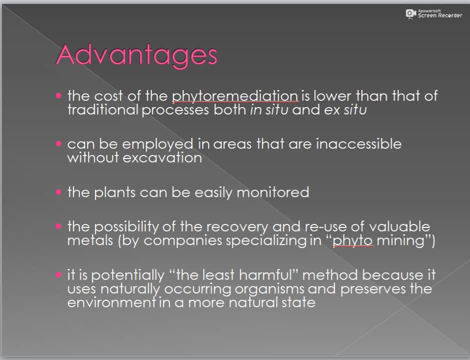 to add one more thing: the all the concepts that we used in the common technique of bioremediation, like uh, bioventing, biopiling, excavation and all that that also can be utilized here in the technology, so you can combine it both together and explain the heavy metal bioremediation. 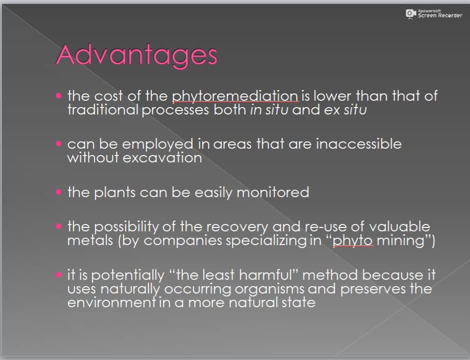 and the bioremediation techniques. so in the previous session i had just given you a common aspect, a common interaction on the bioremediation techniques, and now i just specified what are the mechanisms here by which the heavy metals are being taken up by the plants as well as by the microbes. thank you for now.